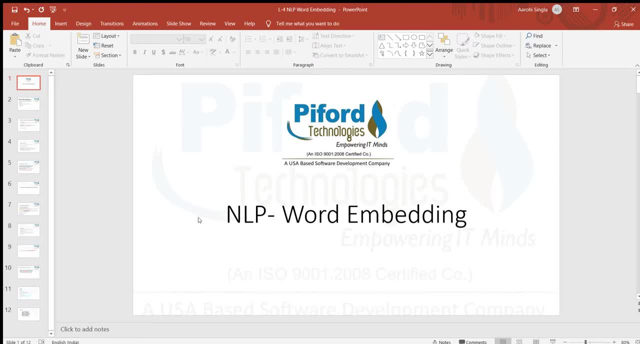 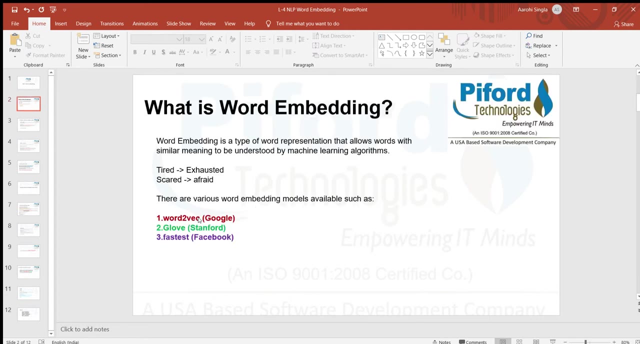 Good evening everybody. this side, Aaruhi from PyFoot Technologies IT Park, Mohali. Our today's topic is Natural Language Processing: Word Embedding. Today we'll discuss about word embedding. So first of all, let's understand what is word embedding, Word embedding simply. 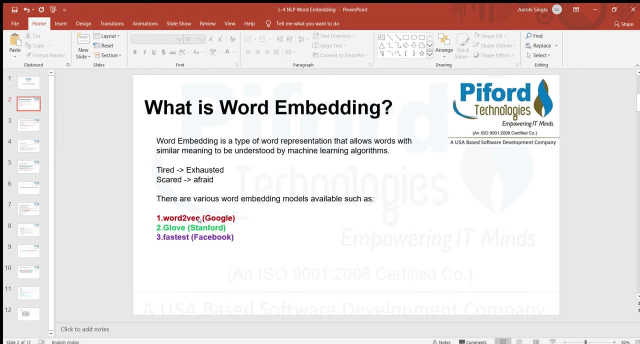 means we want our machine learning algorithms to understand the words which have similar meaning Right. For example, tired and exhausted is the similar word. There is another word, scared, and similar word is afraid. So what we want is that our algorithm should understand. 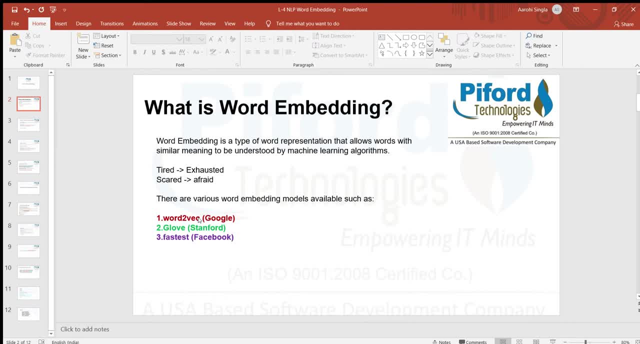 that the exhausted and tired word have similar meaning, Right? So this is what word embedding is. So there are various word embedding models which are available these days. So Word2Vec is a model which is developed by Google For word embedding, and there is another model with the name of Glow, which is developed by 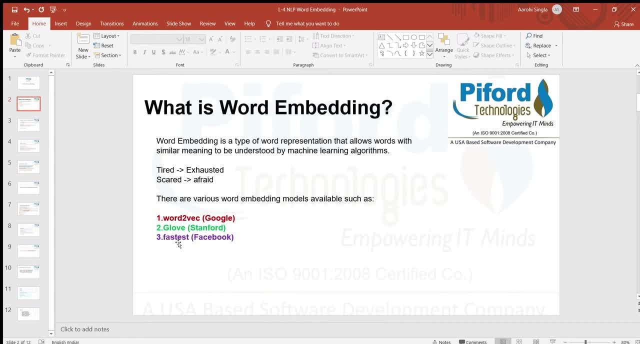 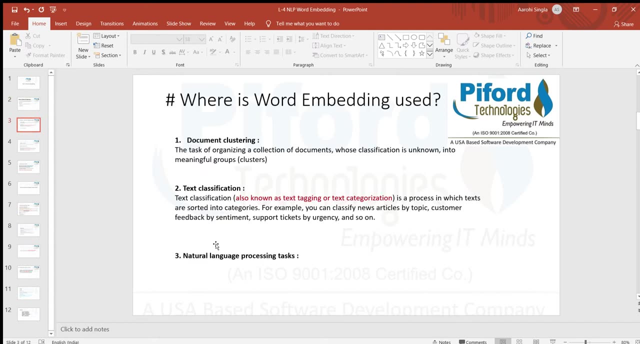 Stanford University. We have another word embedding model with the name of Fastest, which is developed by Facebook. So these are the various word embedding models which are responsible to find out the similar meaning. Now the next question is: where is word embedding used? 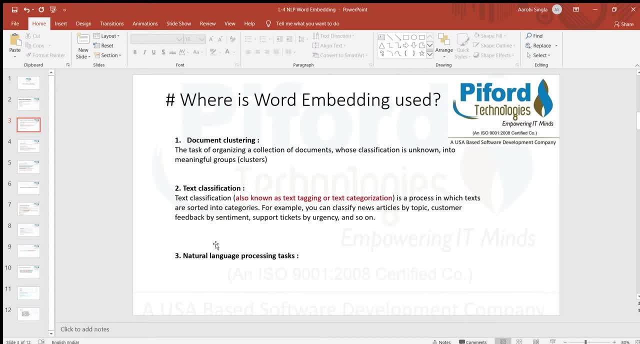 Where we can use this word embedding. So the answer is document clustering, Right, So what is document clustering? So first of all, let's understand what is clustering. So, as you have studied in your previous classes also, So clustering simply means when we have input and we don't have output for that. 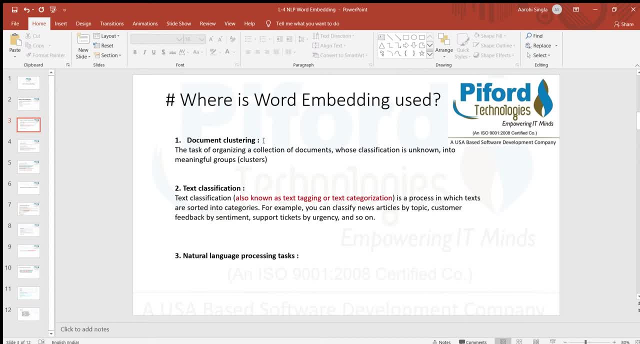 particular input Right And on the basis of similarity we want to group, we want to cluster the elements, input elements Right. So in the case of document clustering, document clustering simply means we want to- let's suppose we have lots of documents Right And we don't know what those documents are Right And 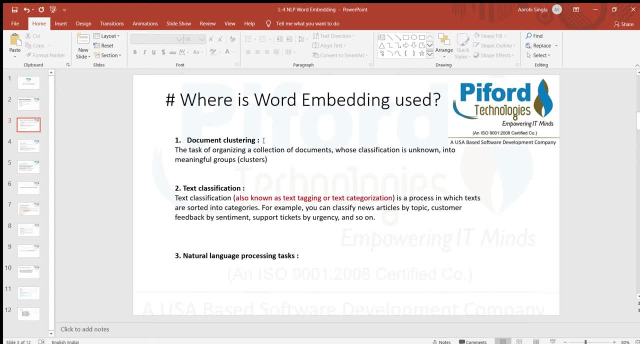 then what we can do is we can cluster those documents on the basis of their similarities. Right, This is one task which we can perform with the help of this word embedding, And the another task is text classification, So classification. Classification belongs to supervised learning, And what does classification So classification? 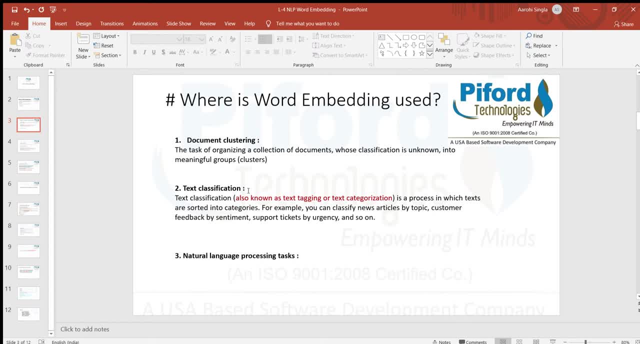 simply means splitting data into predefined classes, Means we already have output classes and we want to split our input data into those predefined classes. So text classification simply means we want to classify the text in predefined classes. Right, For example, we can classify news articles by topic or columns. 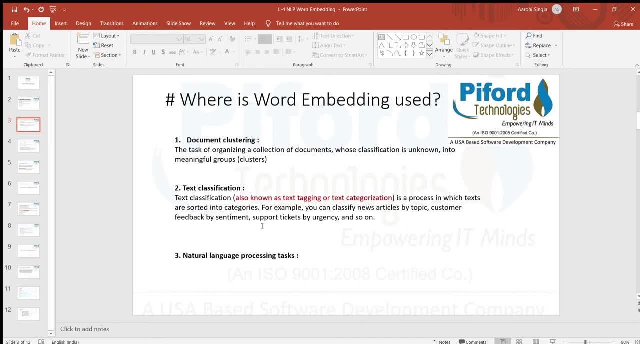 Or customer feedback by sentiment, or we can classify support tickets by urgency. So these are few examples of text classification which we can, you know, which can be done by using this word embedding Right, And the other thing which we can perform with word embedding. 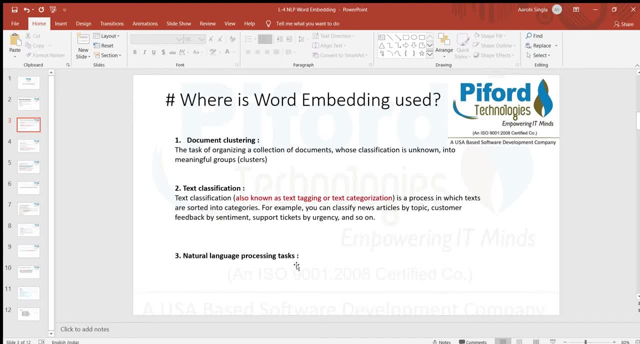 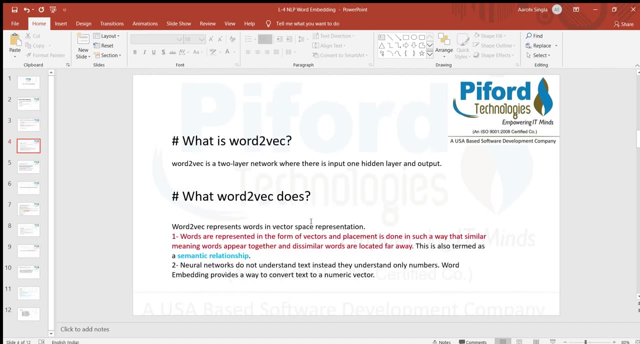 is natural language processing task. So example of NLP is just like key. let's take example of sentiment. analysis Means whether the particular tweet is positive, negative or a neutral. such task can be performed by word embedding Right Now, what is word2vec? So in our 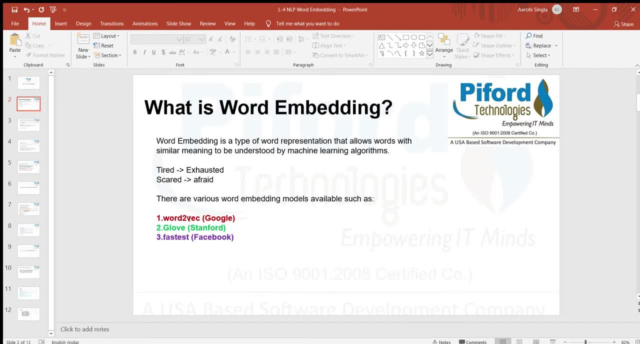 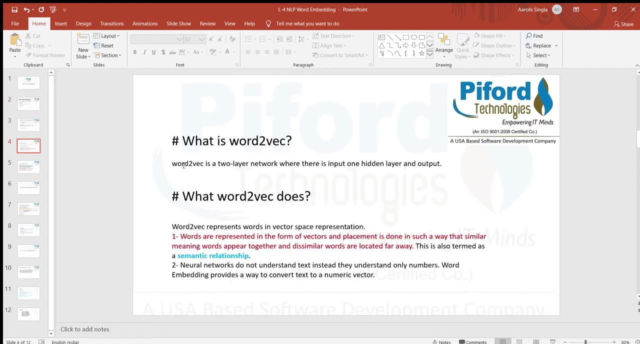 very first slide, I have told you like word2vec is a model which is developed by Google for word embedding task. So in our today's class, I'll teach you how to use this word2vec algorithm, Right? So what is word2vec? Basically, word2vec is a two layer network, Right, Word2vec is? 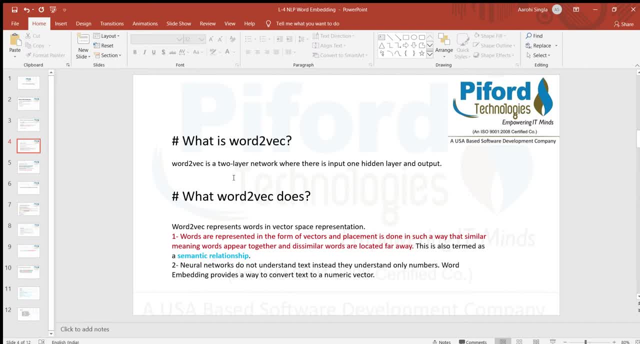 a two layer network simply means we will be having one input layer, one output layer and one hidden layer, Right? So this is what word2vec is, and now let's understand what word2vec does, what it actually does, So how word2vec works Basically, it represented: 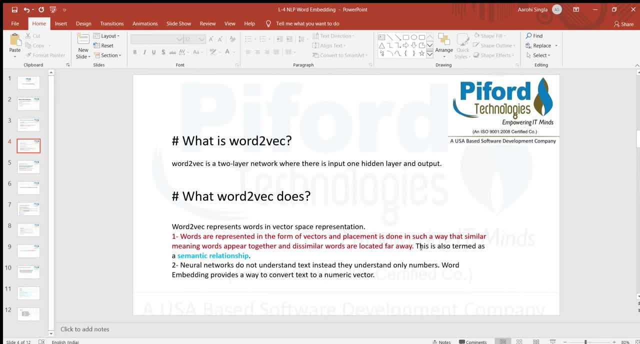 the words in the form of vectors. So word2vec means word2vec represent all the words in the form of vector and means the words which have similar meaning. it will place all those words together and the dissimilar words are located far away. So this is also called semantic relationship. So let's understand. 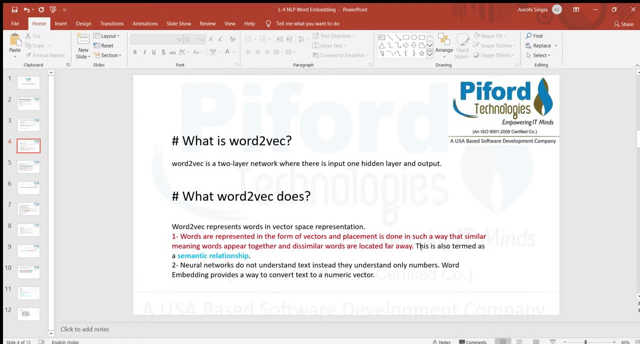 what is the semantic relationship means? Semantic means similar words, Right And word2vec works by grouping all the similar words in one vector and dissimilar words far away from that particular vector. So this is one task of word2vec And another task of word2vec is so as we 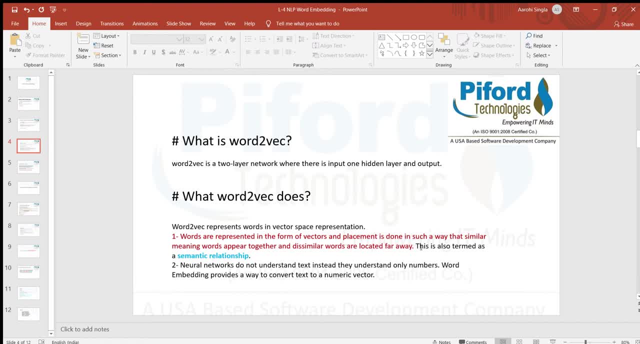 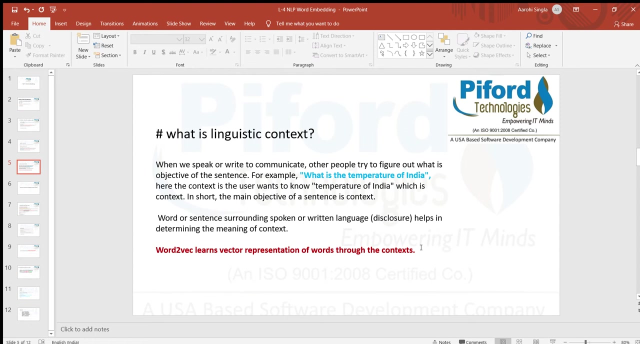 all know machine learning, deep learning algorithms. they don't understand text Right And they only understand numbers. So word2vec. by using this word2vec algorithm, we can convert a text into a numeric vector. So before moving to next topic, I want you to understand the meaning of linguistic context. 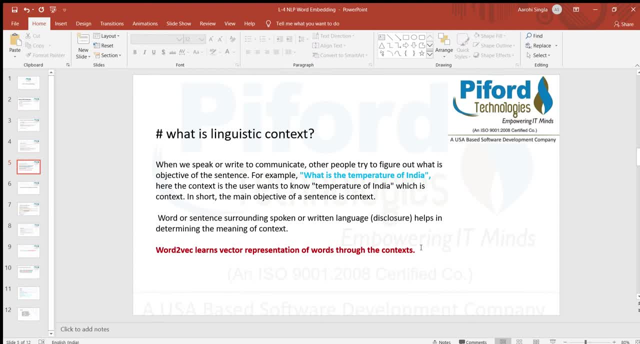 Now, what is linguistic context? Whenever we speak or write something, the other person with which we are talking, that person tries to find, to figure out the objective of the sentence, Right? For example, let's suppose somebody asked me: what is the temperature? 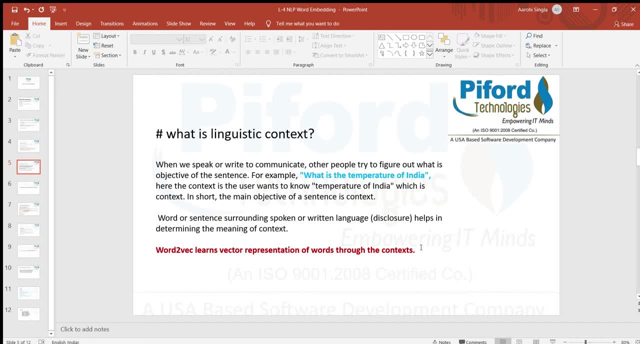 of India. So over here the context is user wants to know about, like what is the temperature of India? So temperature of India is a context in this particular sentence. Right, And word2vec learns. Now word2vec is a model, So model always learn the things. first We train our 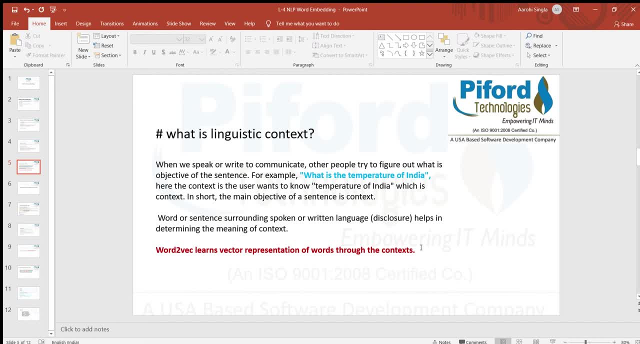 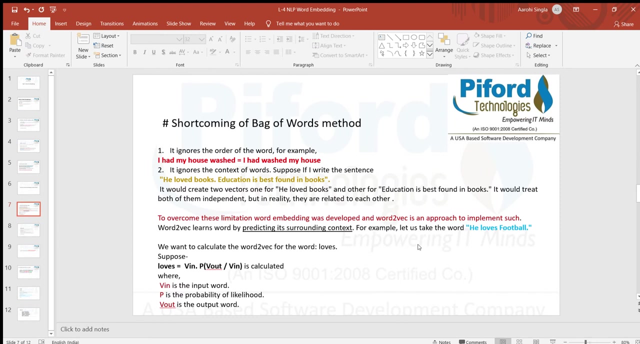 algorithm, then only we can use them for testing purpose, Right? So what is required to train a word2vec algorithm? So basically, word2vec algorithm learns by vector representation of words which have similar meaning Right Now. see, we have studied bag of words Right In a previous class. 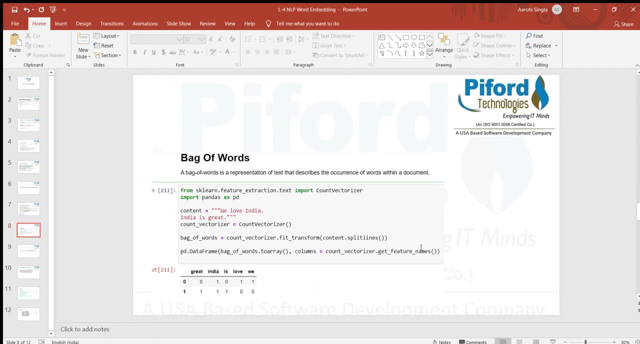 we have studied bag of words, But let me recap the same topic. So let's suppose we have two lines: We love India and India is great, in a variable called contained, And when we applied bag of words on it, So we get this sort of output. So over here you'll see: we love India, India is great. 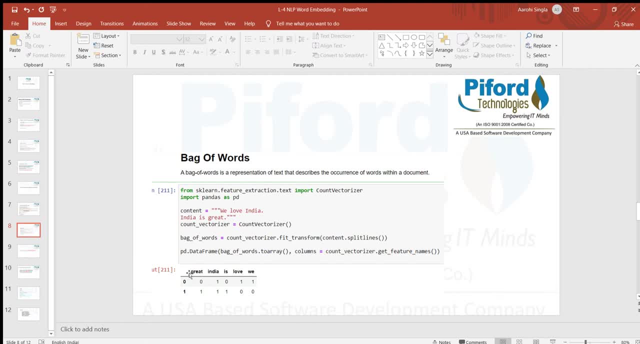 we have that vocabulary over here, but it is not in a sequence, Right, We just have words. So there is no sequence of word And Bag-of-Words is just telling us: okay, a great word is present in a sentence when. 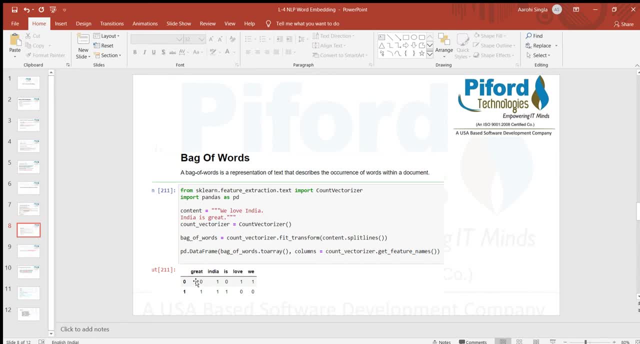 and a great word is not present in the sentence. ah, you know the? in the very 1st sentence great words is not present. and in the next, great word is present. in first, In the next present and in next sentence, great word is present. in the same way again, bag of word is telling us: 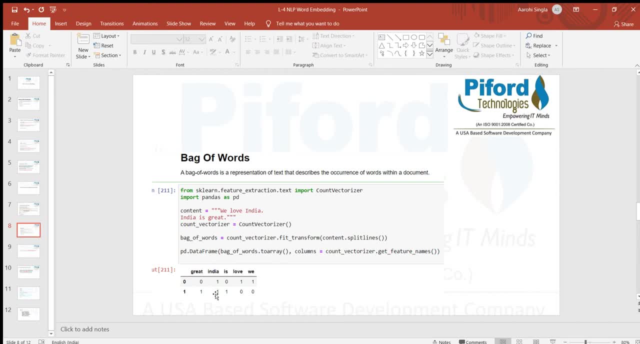 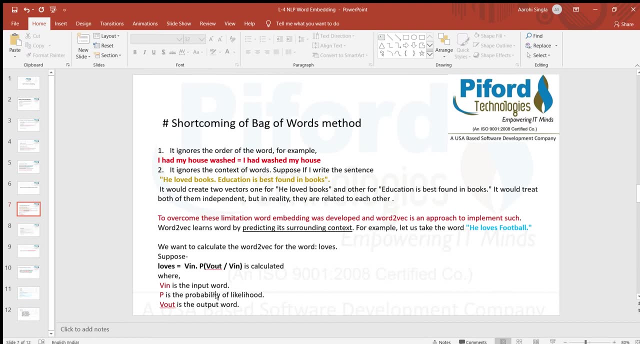 okay, india word is present in both the lines. right, this is what bag of word does. now, the shortcoming of bag of word: it ignores the order of the word means, for example, i have two lines: i had my house washed and another line is i had washed my house. so the words which we are using, 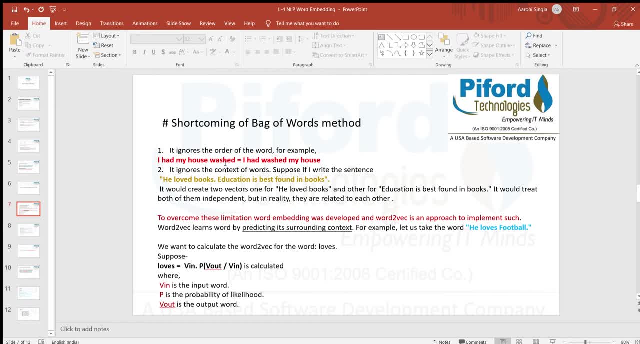 in these two lines the words are same but the meaning is different because of the sequence of the word. so in the very first sentence i am saying i had my house washed means somebody washed my house. and over here i'm saying i had washed my house means i myself washed my house. 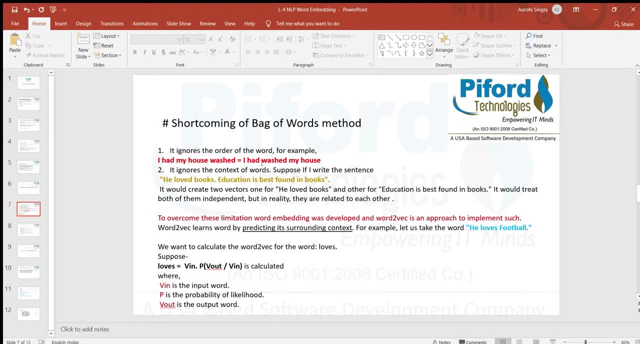 my house, so sequence matters a lot. so these two lines telling us the context is different in these two lines, but when we are using bag of words on it, so that will be a shortcoming because it ignores the order of the word and it even ignores the context of the word, because it will only see like 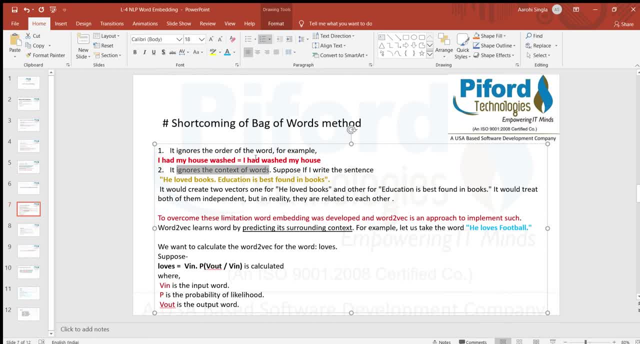 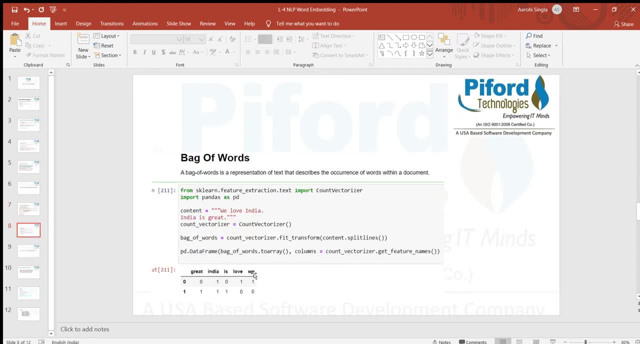 okay, these words are present in this line and these words are present in this line and bag of word is not taking care of a sequence. you can see over here: sequence. bag of word is not taking care of sequence. it is only you know writing the, the word and telling us whether that word is present. 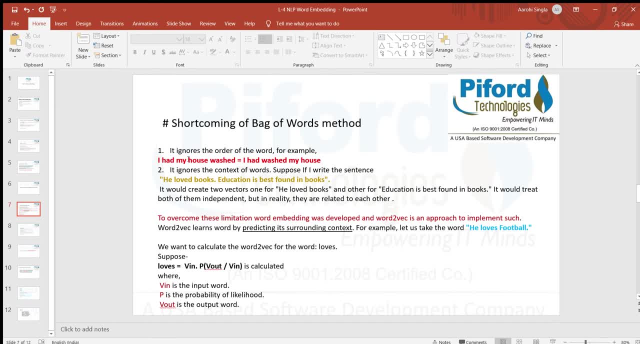 in any particular line, or not, right? so these are the shortcomings of bag of words. but these two shortcomings, you know, word to wick have overcome these two shortcomings. so word to wick. now let's see how this algorithm works, right? so let's understand by one line. so over here i'm using a line he loves. 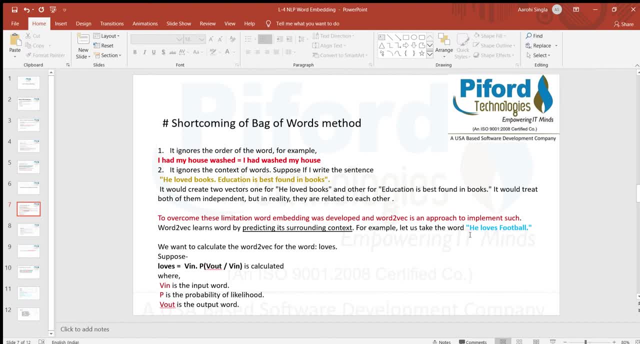 football. so this is a sentence: he loves football and i want to use word to wick model on it. so, first of all, what we will be doing, we will see the word to wick for loves, because the important word over here is loves, right? so let's calculate the word to wick for the word loves. so this is: 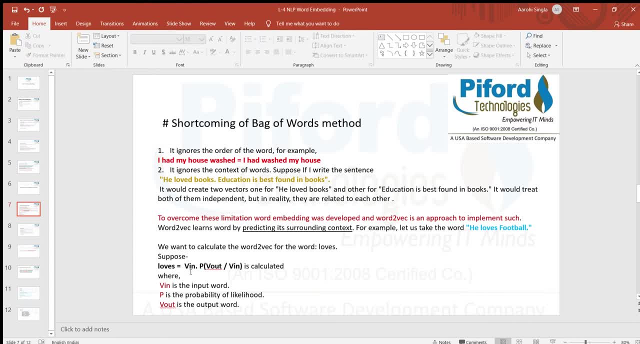 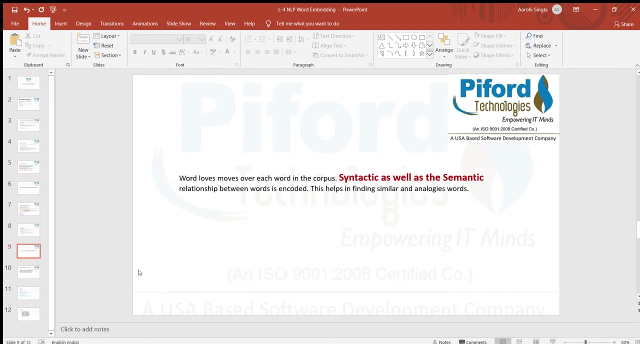 the formula for it. so formula is v in. v in means the input word, dot, p means probability, v out means the output word divided by v in input word, right? so this is the formula which word to wick algorithm follows to solve the problem, right? so basically, uh, so over here i've told you we are calculating. 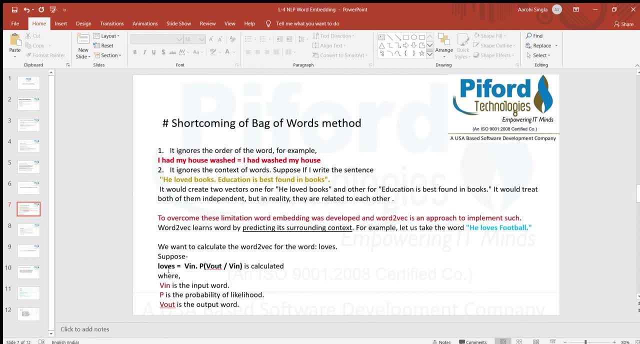 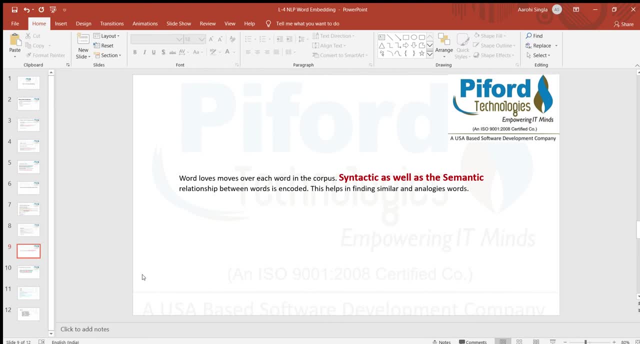 word to wick for love, uh, love's word right. so what will happen is this word loves that particular word. love word will move through the document, means it will move through each and every word of the document and then it will find out syntactic as well as semantic relationship. 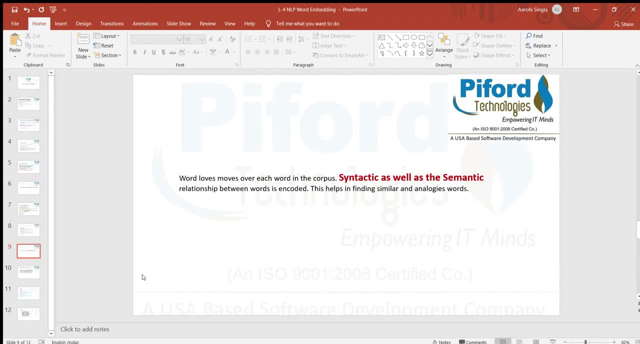 now, what is syntactic? syntactic means sequence of the words and as well as semantic, semantic means similarity between the words. when this lover loves will move through each and every word of the document, it will find syntactic and semantic relationship between the words. this is how the word to wick. 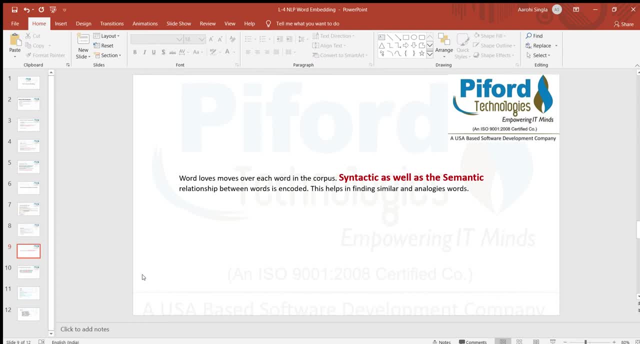 algorithm will display similar words and dissimilar words. so in this whole um lecture we has started understand how to about words by adventure, word to wic, where we can use this word to wic whenever we want to find similar words or we want to find dissimilar words or we want to reduce the dimensions. so we all know dimensionality. 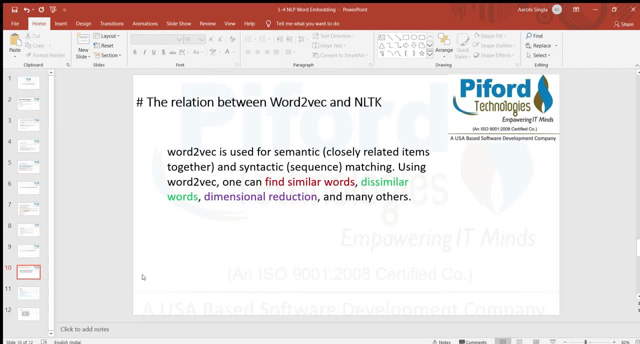 reduction is a very good data pre-processing technique, right? so in machine learning you have studied pca also, by which you reduce the dimensions. so over here we can reduce dimensions by using word to wic also. so these are the few functionalities which we can perform by using word to wic, right? so now i'll share one practical example of finding similar words. 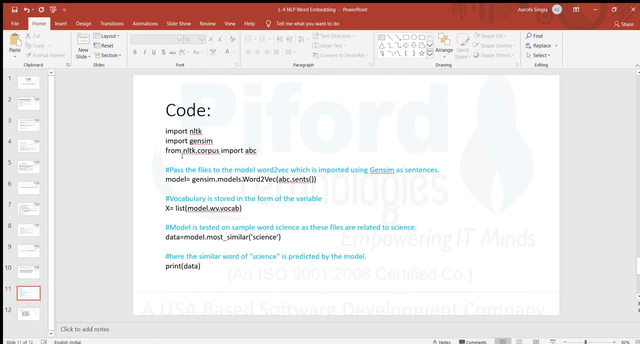 right. so this is the code of that particular code. so right now, first of all i'm importing all the required modules and then i have a variable with the name of model. in this model variable i'm calling this gen sim. gen sim is a module for nlp. so from gen sim i'm importing all the modules and from those modules i'm using. 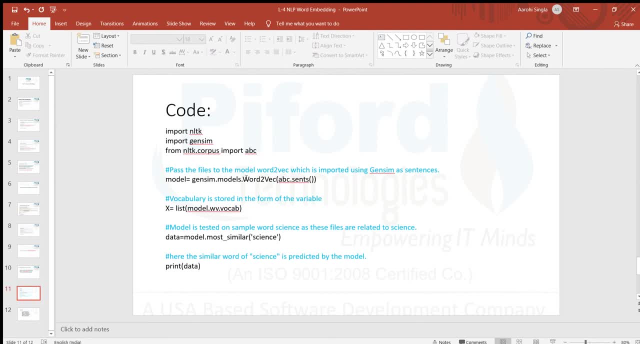 word to wic module means this word to wic module as lying in this gen sim module. so that's why we are importing it. so and then abc dot sense. so over here you'll see from nltk dot corpus import abc. basically abc is a corpus. what is corpus? corpus simply means: 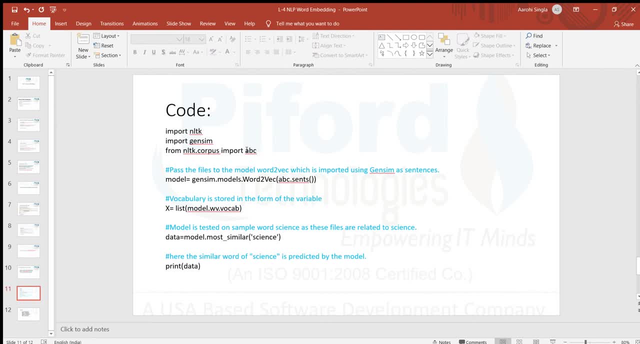 a collection of text, lot of text, right, collection of lot of text. so there are lots of corpus in nltk, so over here i'm importing abc. corpus means there are lots of text which lying under abc, so i'm using that right abc dot sense. sense means sentences. i want to import all. 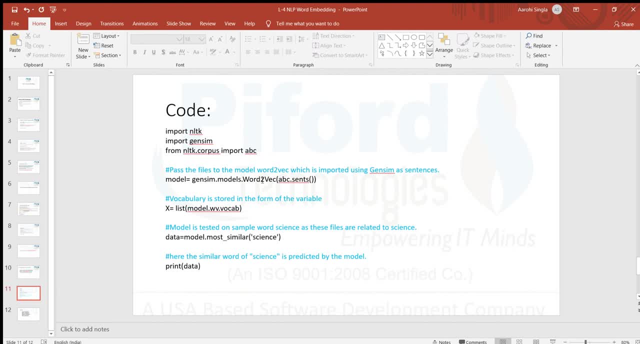 the sentences which are present in abc, and i want to apply word to wic on it, right? so that's why we are importing it and storing that result in a model variable. now, in next variable, in x variable. what i'm writing over here is model model. is this variable which? 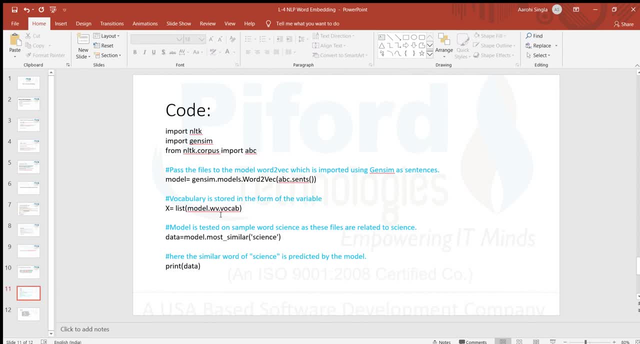 is carrying this whole task: dot we, dot vocab. now i'm getting all the vocabulary which is present in abc and storing all that vocabulary in x, because on the basis of this vocabulary we will further solve our problems. now i have another variable with the name of data and